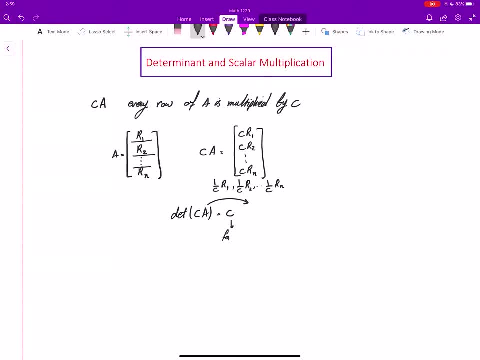 so it will give us c for row 1.. This another c, row 2, another c, row 3, and so on up to row 3.. and how many of these? we have N of them. Then the matrix. well, let me just then draw this. 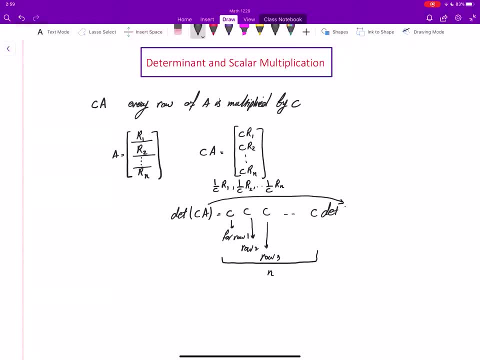 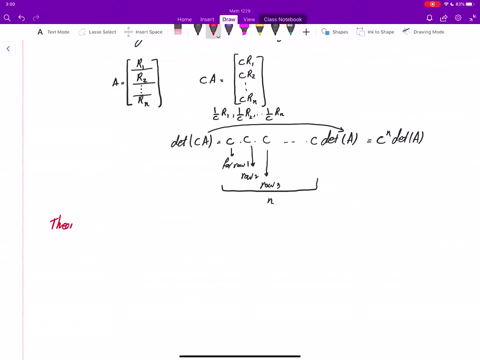 row operation as we have. this is A. How many of these guys? we have N of them. It means that we have C and the determinant of A. So when you multiply, this is a fact. now this is a theorem. I just proved it for you. For a square matrix, let A be an N by N matrix. Then 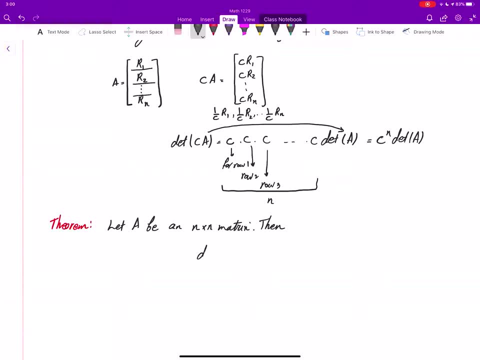 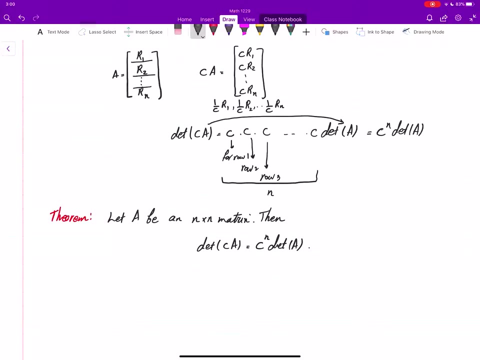 determinant of C. A is not just C. determinant of A. This is C to the power N. The number of rows: The number of rows appear there as the power of C. Okay, So that's the property: How scalar multiplication changes. determinant by a constant C to the power N. Let's do some examples here. 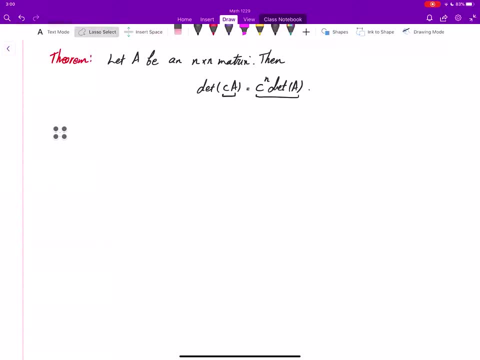 Just yes. okay, Here I have a two by two matrix whose determinant is three. What's the determinant of five A? Well, this guy, you have five times A. This, in other words, this is C, And we know that scalar multiplication to come out of the determinant. 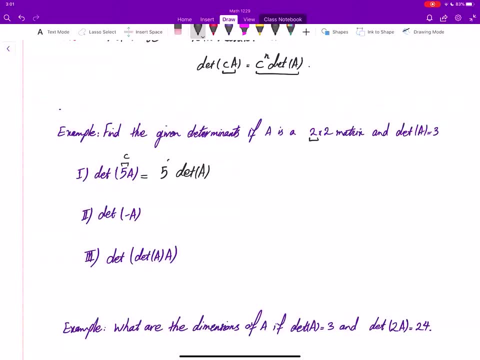 you have to put the number of rows as power of that scalar. So this is 25.. Determinant of A is three, So three times 25 is 275.. Okay, How about determinant of negative A? Well, negative A is same thing as multiplying negative one. 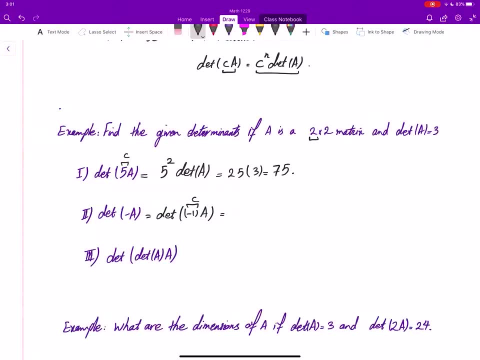 to A. Yes, So that is C here. So then negative one to the power two comes out. This is determinant of A, And we know that negative one to the power two is just one times three gives us. How about this? one Determinant of A times A. 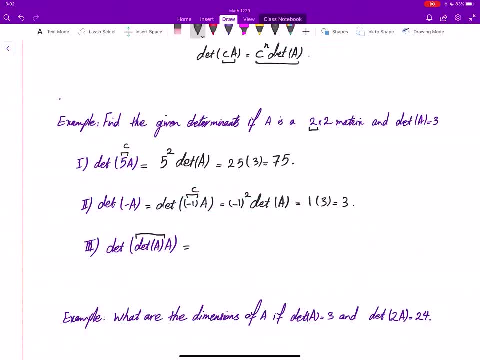 Okay, How about this one Determinant of A times A. How about this one Determinant of A times A? Okay, You see, determinant of A is a number, So we can take it as this scalar that we are multiplying to A. And we know that scalar comes out of determinant, whatever C is. but we have to put 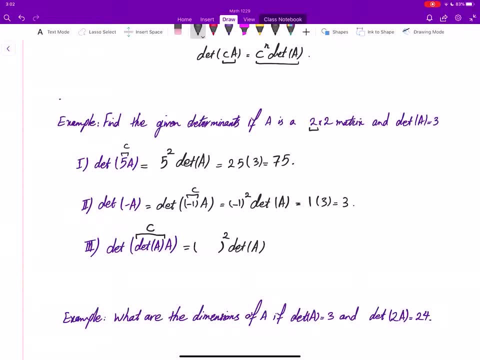 it in the power two. Well, here C itself is determinant of A. In other words, we have determinant of A to the power two. Okay, So we have determinant of A to the power two. Okay, So we have determinant of A to the power two, times determinant of A, which is determinant of A to the power three. So, 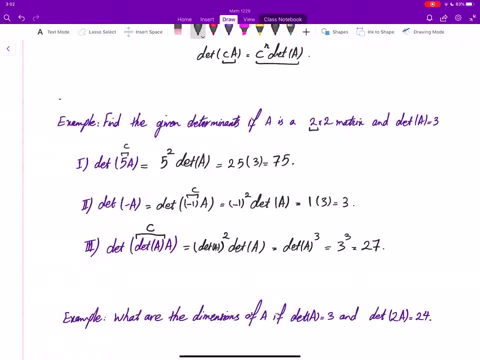 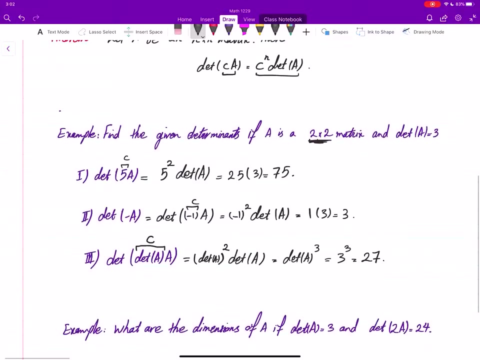 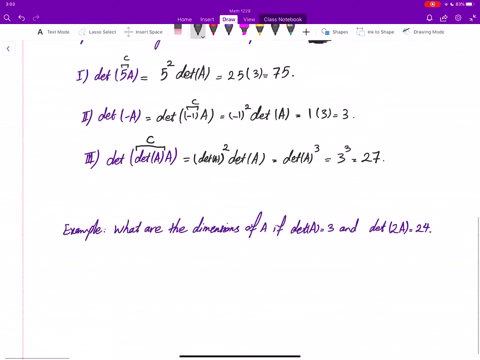 three to the power three, which gives us 27.. Without knowing the dimension of matrix, you cannot say what is determinant of five A just by knowing determinant of A. You need to know what is that N, otherwise the formula doesn't work. And that brings us to the next and last example, which 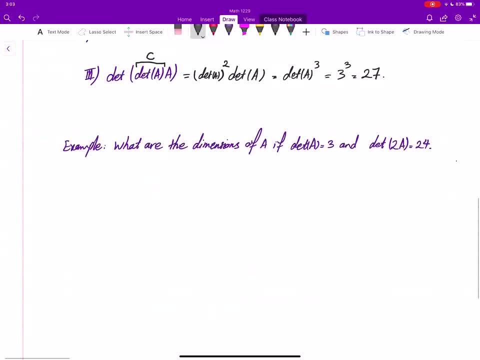 says: okay, if you know how determinant changes in the scalar multiplication, you might be able to find the dimensions of the matrix. So here, determinant of A is three and the determinant of two A is 24.. Well, determinant of two A is 24.. But what we know is that determinant of two A 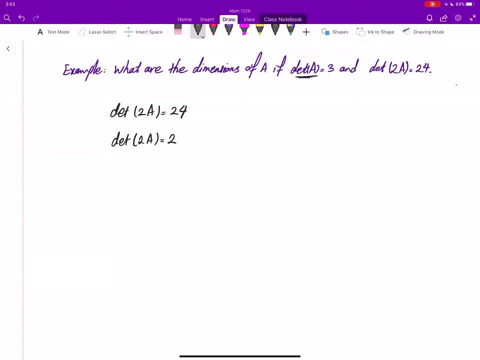 is equal to two to the power. whatever the dimension of this number of rows, of this matrix, A is and times determinant of A. In other words, we have two to the power, N. well, determinant of A is what Three. This is going to be equal to 24..